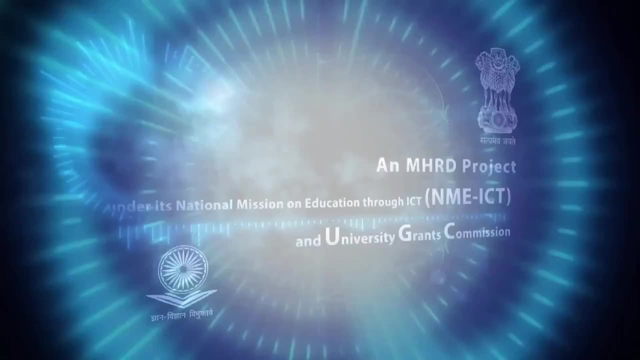 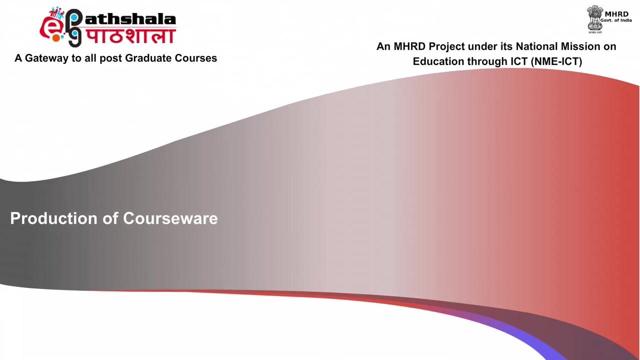 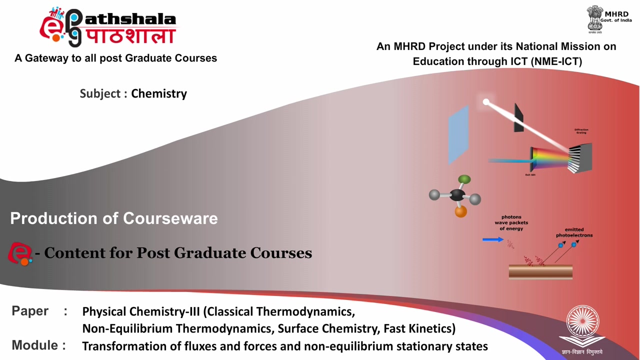 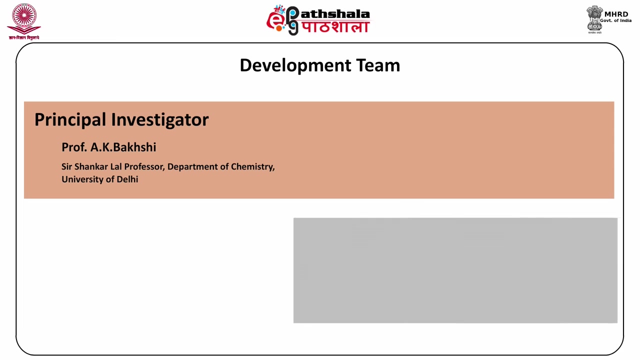 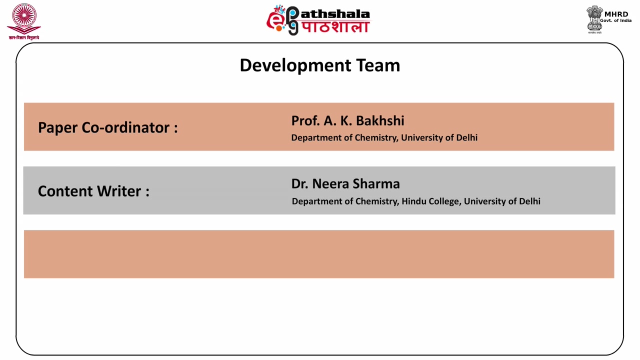 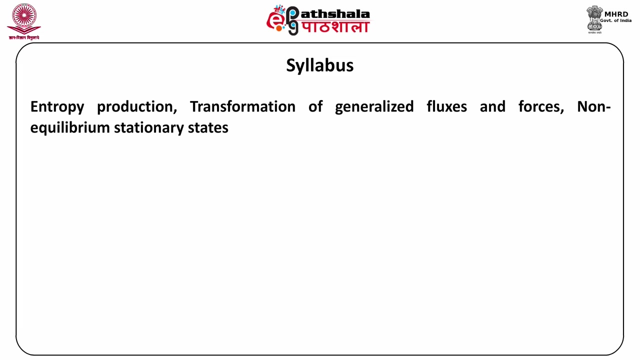 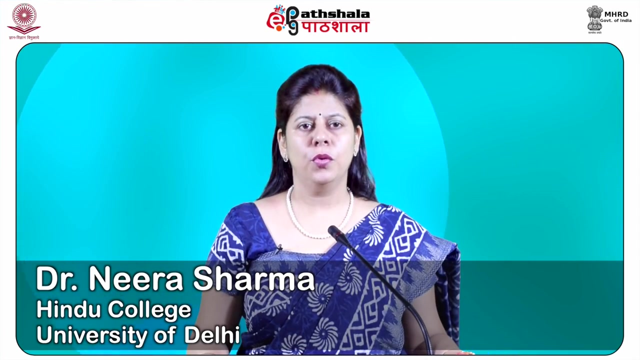 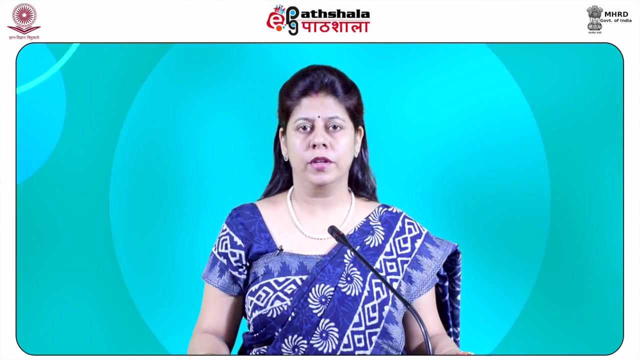 Thank you for watching. Thank you for watching. After studying this module, you shall be able to know about the entropy balance equation, learn how the entropy production is related to affinity of the reaction, learn how the fluxes and forces are transformed and about non-equilibrium stationary states. briefly, 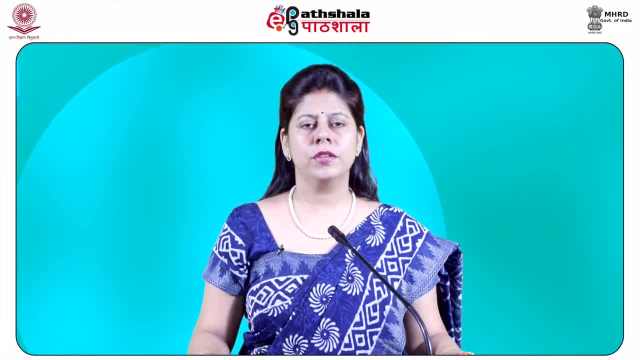 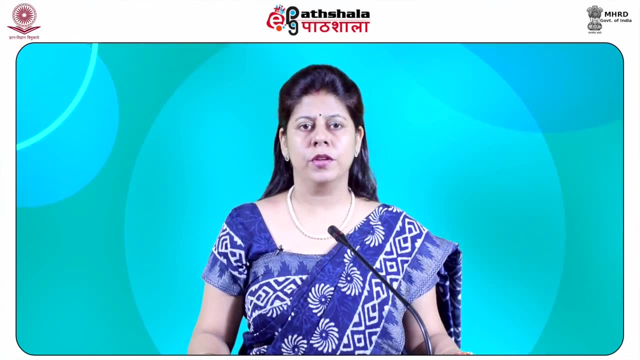 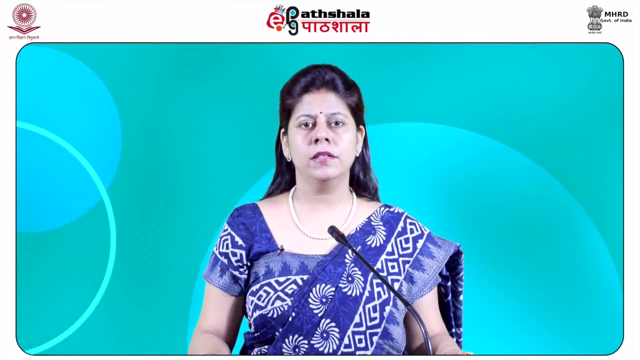 Entropy balance equation. The basic equation for non-equilibrium thermodynamics is entropy balance equation. This balance equation for entropy can be derived using the concept of conservation of energy and the balance equation for the concentration. This equation depicts the relationship between three thermodynamic quantities. They are: the entropy change, the 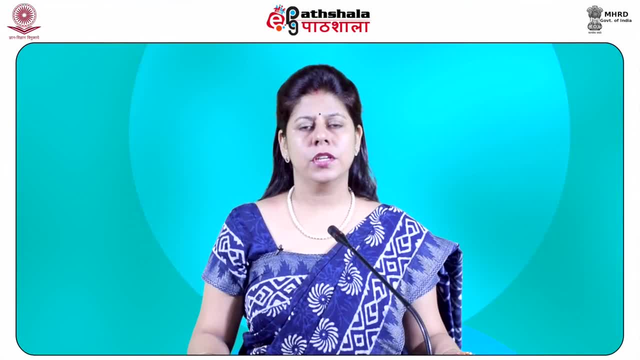 entropy production and the entropy flow. The change in entropy is the time derivative of the entropy of the system. The change in entropy is the time derivative of the entropy of the system and it is the sum of two integrals- entropy production and entropy flow- for a. 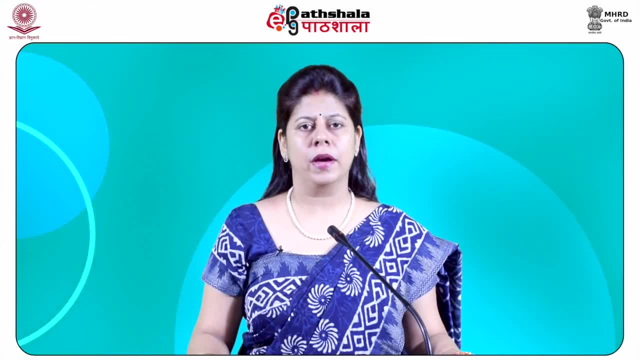 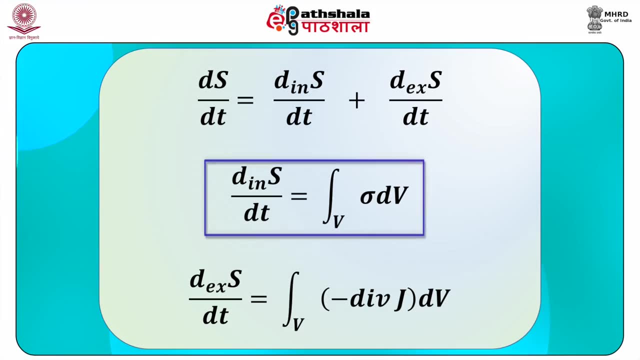 given system And the expression is given by ds. internal, by dt, denotes the entropy production and is written by the integral of sigma into dv. This time derivative of entropy denotes the entropy produced within the system. The time derivative of external entropy is the time derivative of internity in the system. The change in entropy is the time derivative. 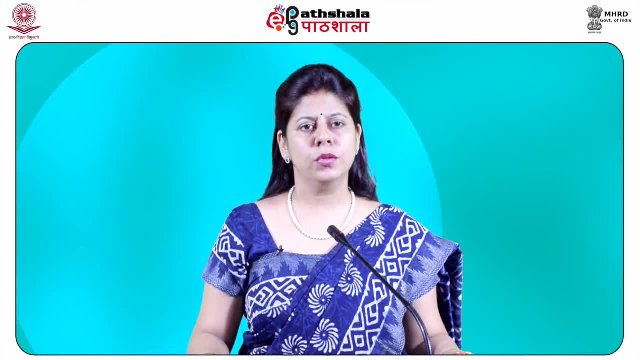 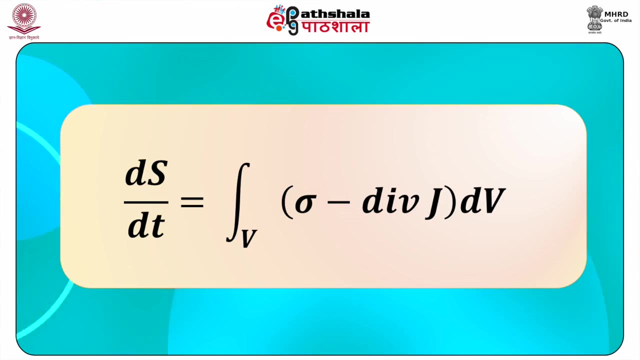 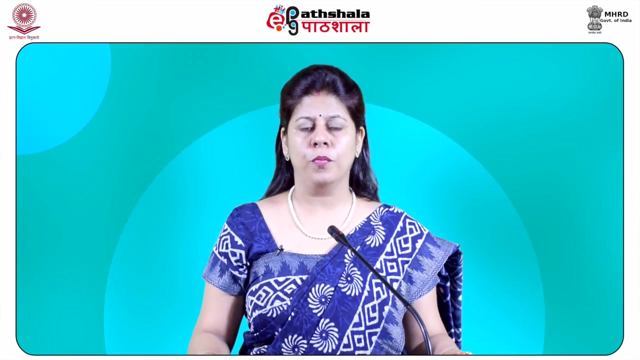 generated at d1 of Rn. from Rt to R dP, The change in energy production is given by the integral sigma Qing. Hello, welcome viewers. Here I am Sonali. I will be conducting session on change of energy of J into dV For a reaction diffusion system. the entropy production comprises of two components. 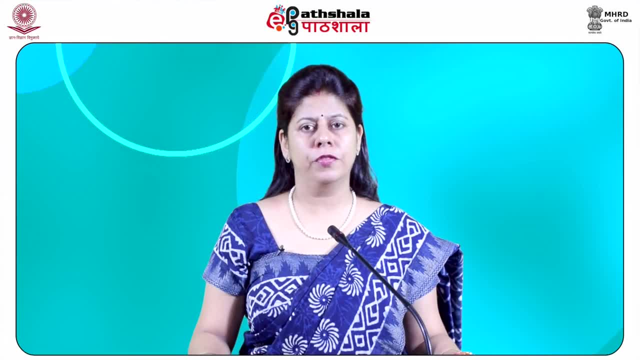 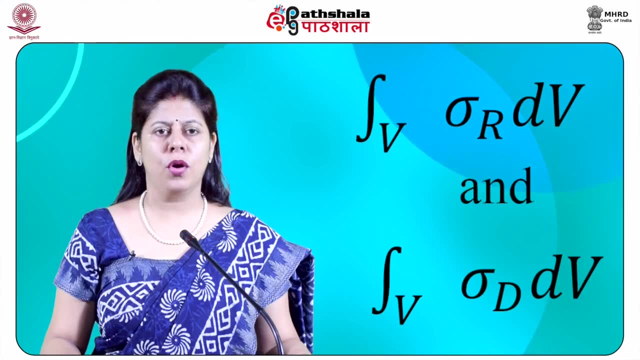 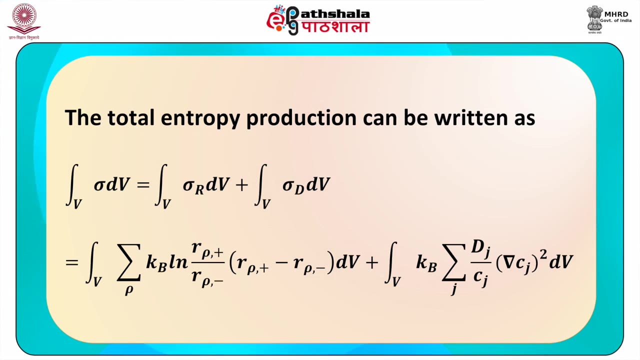 the entropy production of chemical reactions and diffusions respectively. The total entropy production can be written as the sum of sigma R, dV and sigma dV. From the above expression you can see that kB denotes the Boltzmann constant, rRho plus and rRho minus represents 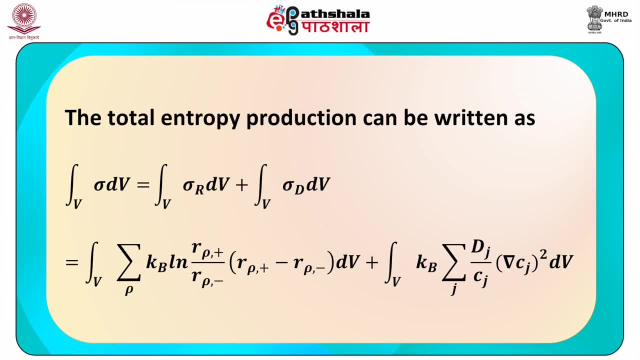 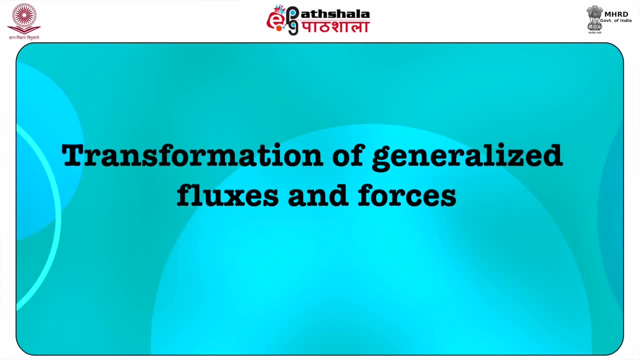 the rate of forward and backward reactions of the row earth. chemical reaction. dJ and cJ represent the diffusion coefficient and the concentration of the jth component respectively. Transformation of generalized fluxes and forces. The rate of entropy production for an irreversible process. software's experimental configuration provides the following information: 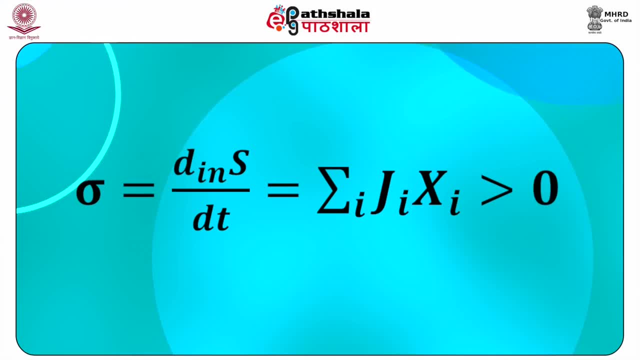 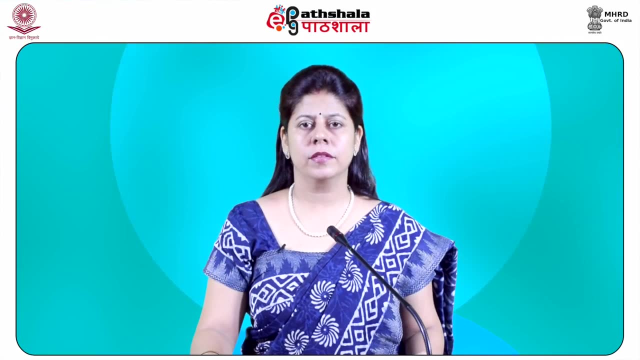 is given by the summation of Ji into Xi, which is greater than 0.. For a single chemical reaction occurring at a given rate, the above expression can be written as the product of J and X. Sigma does not depend on the reaction sequence, but depends on the linear combination of forces. 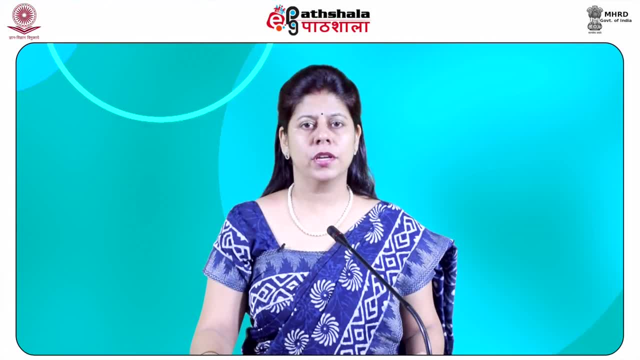 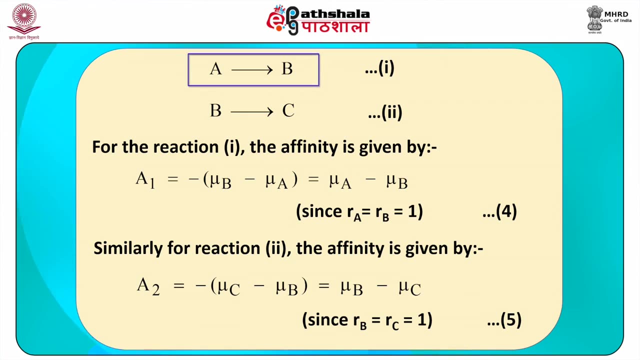 and flows. In the above equation the flux J is identified with the rate R and generalized forces X is identified with the affinity. Consider a consecutive type of reaction in which A gives B and in the second reaction B gives C. For the reaction 1, the affinity. 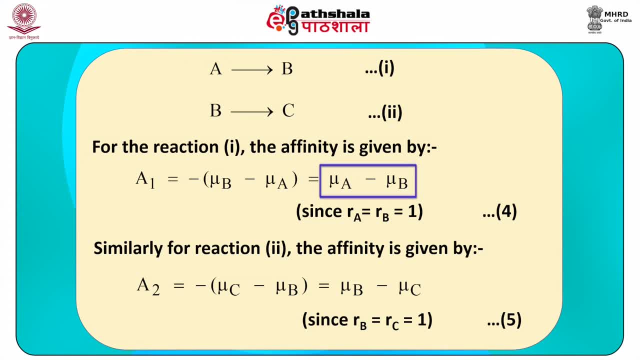 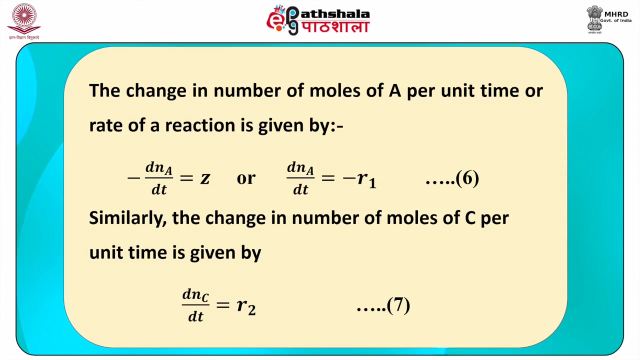 is given by the difference of MuA-MuB, Since Ra is equals to Rb is equals to 1.. Similarly, for reaction 2, the affinity is given by MuB-MuC, since Rb is equals to Rc, which is equals to 1.. The change in number of moles of A per. 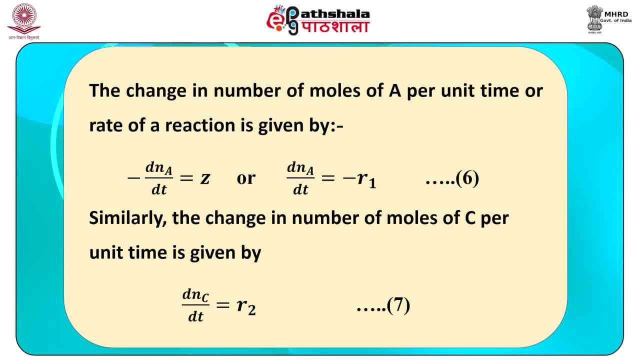 unit time or rate of reaction is given by dNa by dt, is equals to minus R1.. Similarly, the change in number of moles of A per unit time or rate of reaction is given by dNa by dt is equals to R2.. 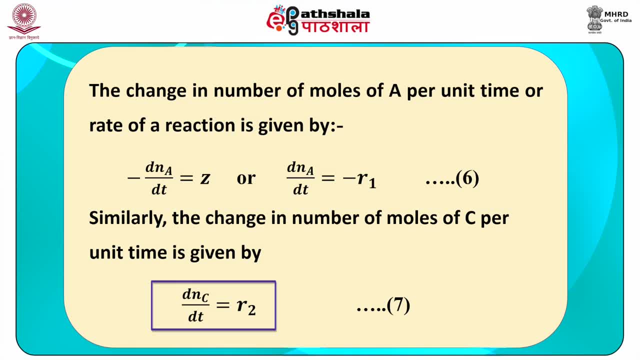 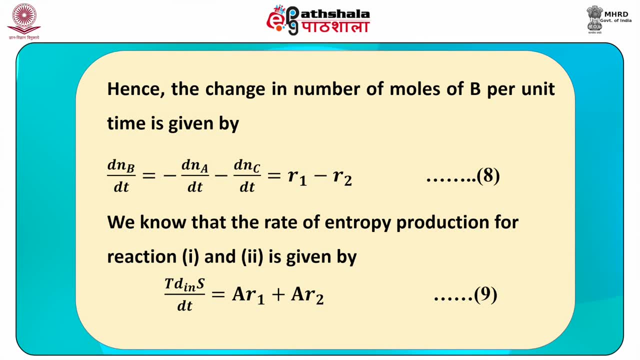 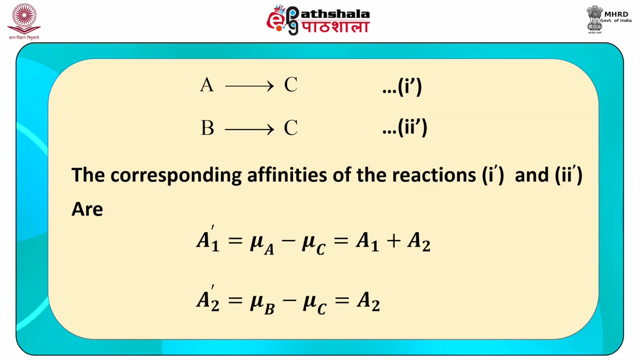 Since B is equals to R0, the tangent chegable is given by R1.. S we know that the rate of entropy production for reaction 1 and 2 is equals to R1, A2 plus A2.. Now consider a different chemical reaction in which A gives C and B also gives C, The 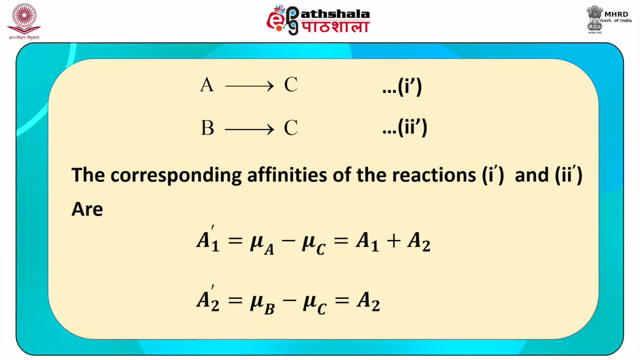 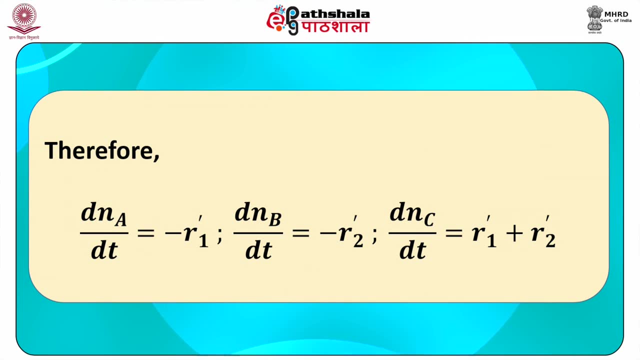 corresponding affinities of the reaction. 1' and 2' are: for A1' it is equals to A1 plus A2, and for A2' it is equals to A2.. Therefore, the change in number of moles of C is equals. 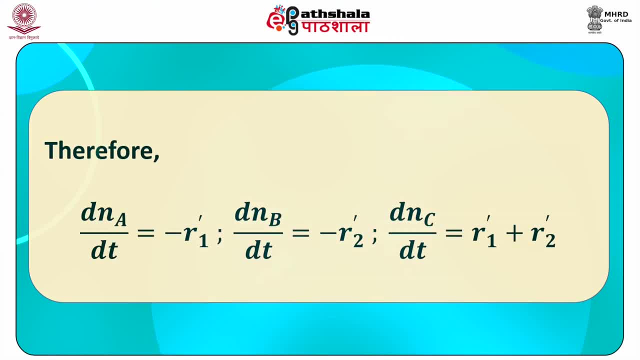 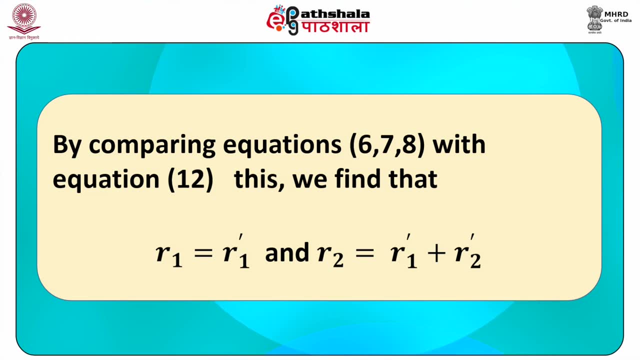 to R1' plus R2' By comparing equation 6,, 7, 8 with equation 12, we find that R1 is equals to R1' and R2 is equals to R1' plus R2'. For this reaction, the rate of entropy. 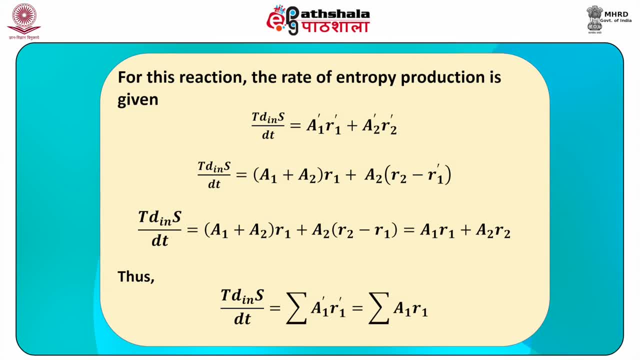 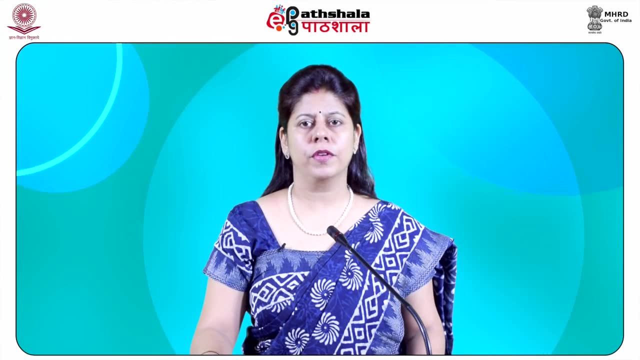 production is finally given by equations, which is the summation of A1' into R1' plus R2', which is equals to summation A1 into R1'. The above equation suggests that the newly generated set of equations for entropy production are also same. 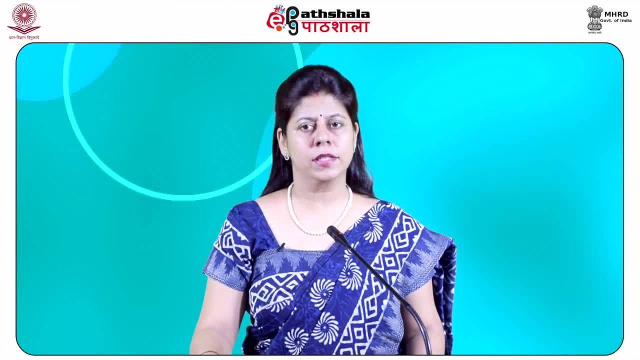 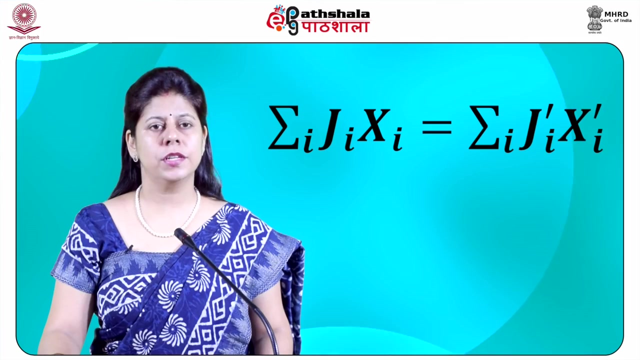 Thus the transformation properties of the fluxes Ji and the generalized forces Xi are such that linear combination of forces and fluxes give a new set of fluxes Ji' and a new set of fluxes Ji''. Thus the equation holds good. Therefore we have summation Ji. Xi is equals to summation. 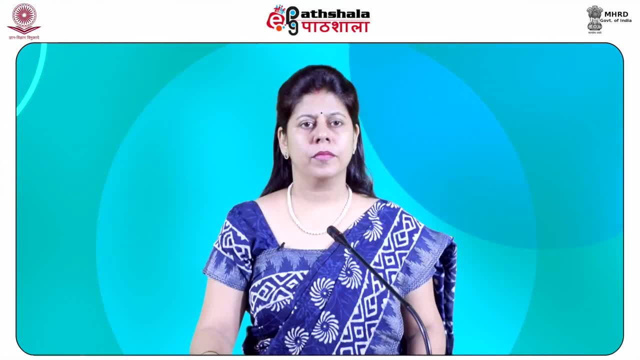 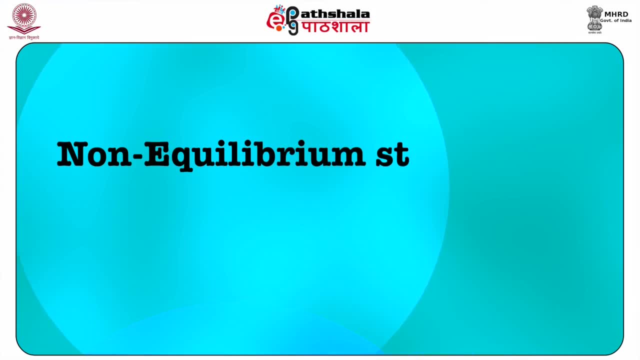 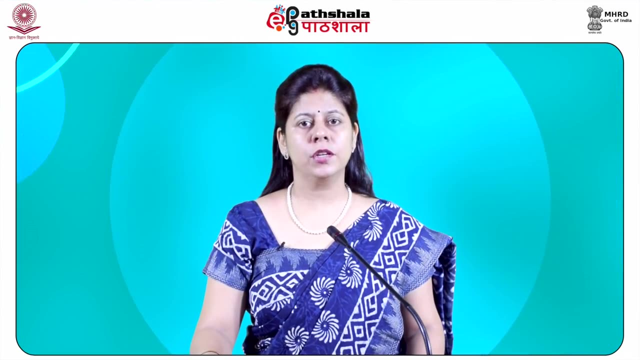 Ji' into Xi' There are three types of transformations in linear irreversible thermodynamics. Now we will discuss about non-stationary states. Non-equilibrium stationary states are the state variables which are non-equilibrium. Non-stationary states are the state variables which are independent of time, In this case, entropy production is different from 0, and there is no transport of mass, ie the Jm is equals to 0. Whereas equilibrium states are the states in which entropy production is 0.. A stationary state arises when the concentration of the intermediate components does not vary. 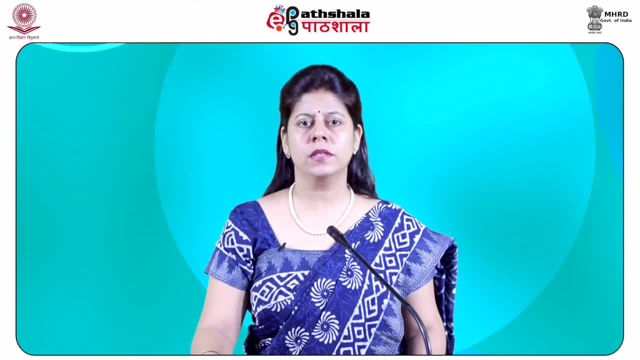 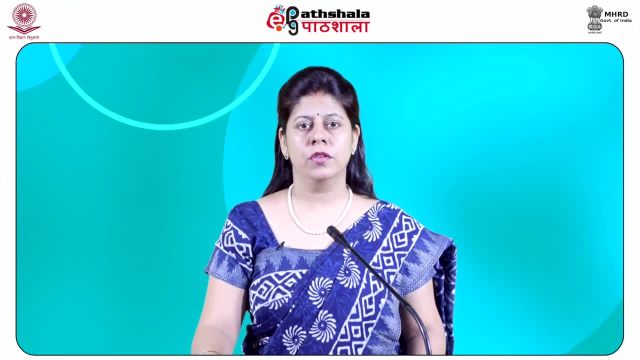 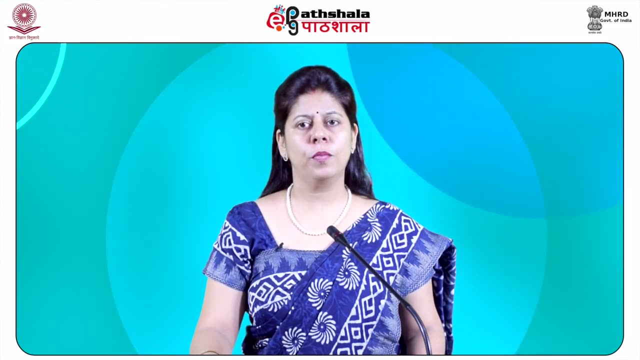 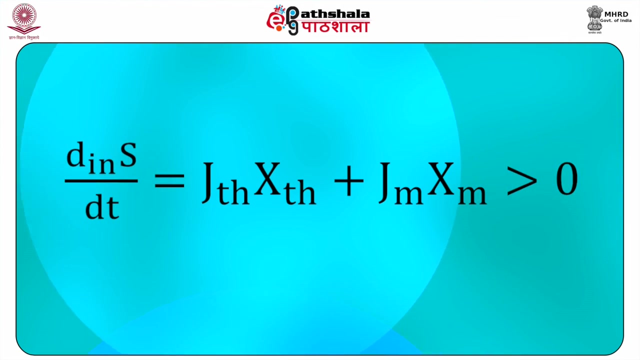 with time, one component system in which there exist temperature gradient as well as the concentration gradient, which are denoted by Xth and Xm respectively. Near equilibrium entropy production per unit time can be written as the sum of Jth, Xth plus Jm, Xm, which is greater than 0, and the 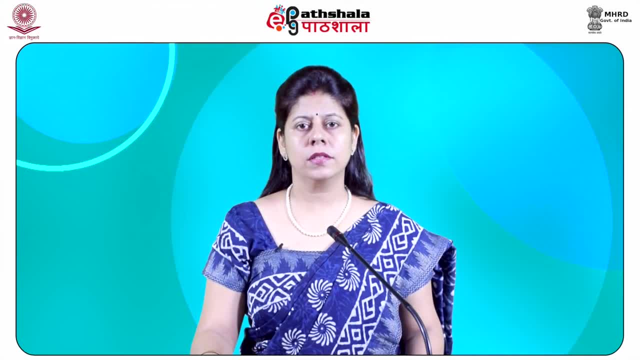 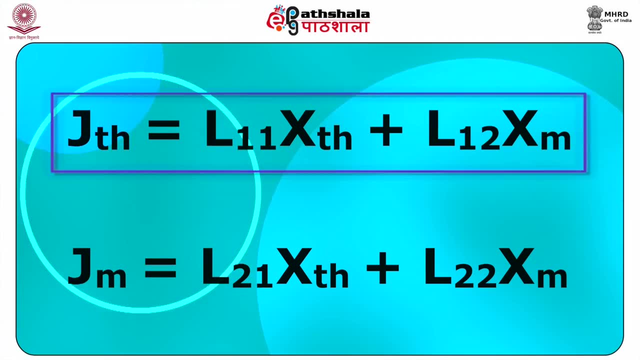 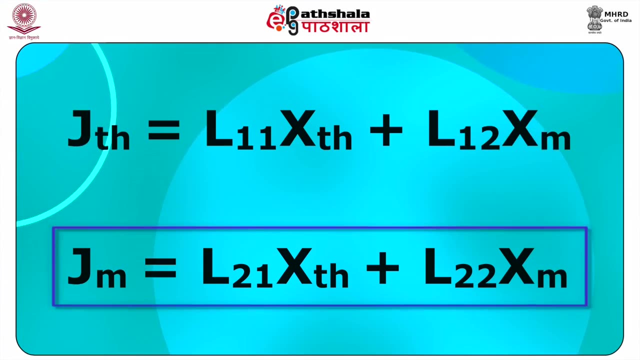 linear phenomenological laws which we will discuss later are: Jth is equals to L1 Xth plus L12 Xm, and Jm is equals to L21 Xth plus L22 Xm, where L11 and L22這些重點計 和加重的發電 revenge coefficient of thermal conductive and diffusion coefficient. 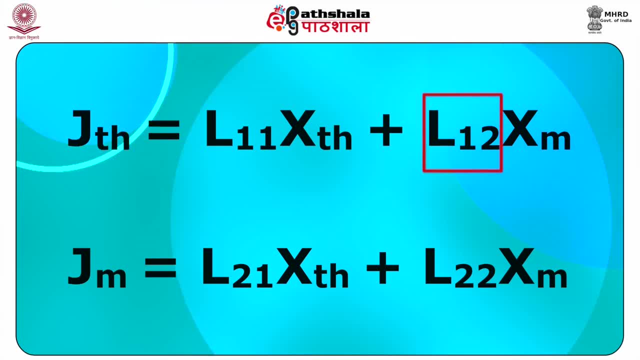 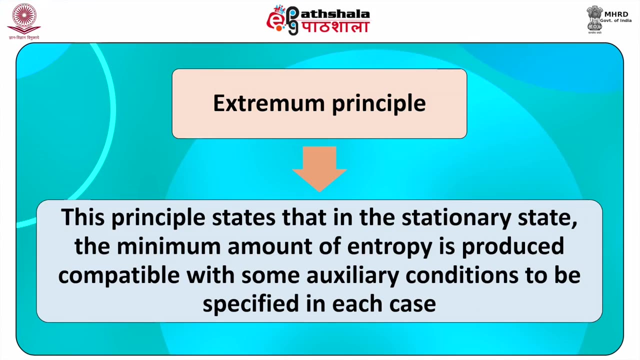 R receiver. L11 and L22 are the coefficients of thermal conductivity and diffusion. coefficient, respectively, is the coefficient of heat flow related to a concentration gradient. L21 is coefficient of mass flow associated with a temperature gradient. Stationary states may be characterized by extremum principle. This principle states: 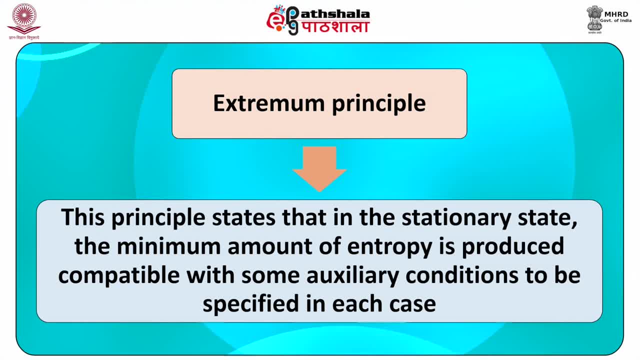 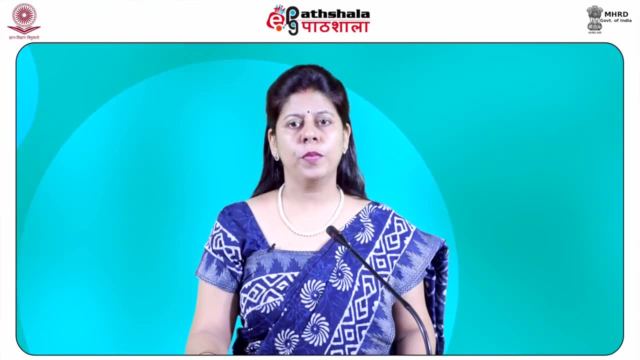 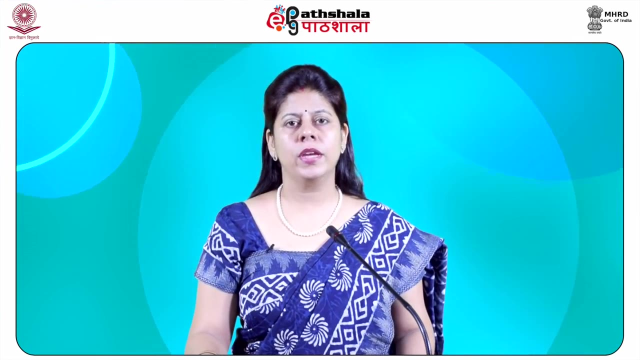 that in the stationary states the minimum amount of entropy is produced, compatible with some auxiliary conditions to be specified in each case. Thus an equation may be derived that specify conditions that entropy production has minimum value for a given value of Xth. Thus, using equations and on Sager reciprocal relation, which is L12 is equals to L21, the 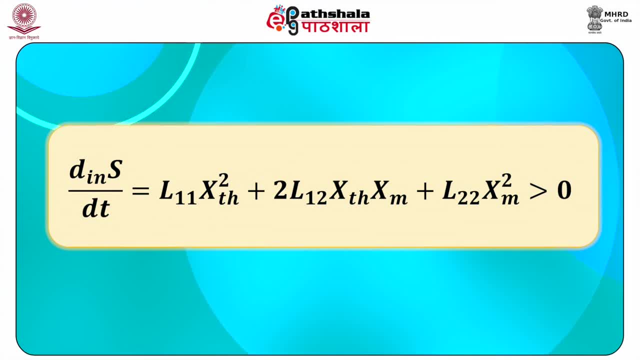 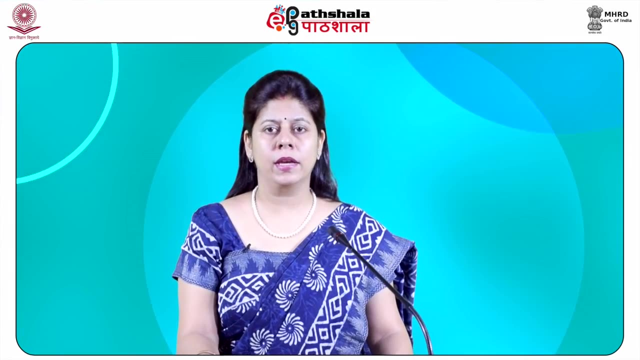 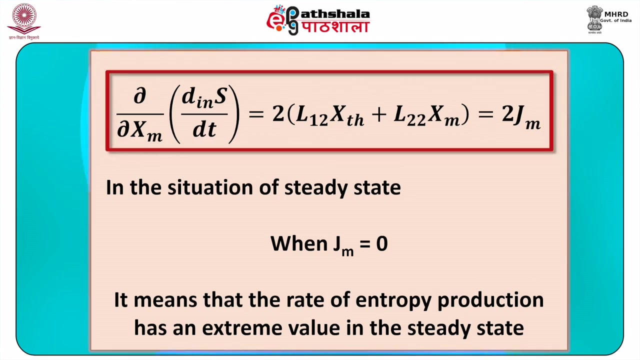 rate of entropy, production becomes L11 Xth square L21.. Taking the derivative of equation 19 with respect to Xm, keeping Xth constant, we get twice of L12 Xth plus L22 Xm, which is equals to twice of Jm. In the situation of steady, 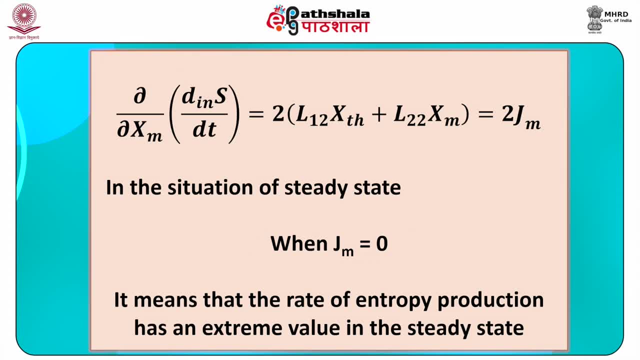 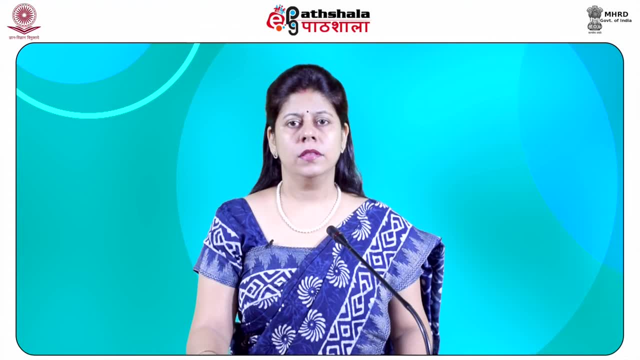 state, when Jm is equal to L22 Xm, we get twice of L22 Xth plus L22 Xm. In the situation of steady state, when Jm is equal to zero, it means that the rate of entropy production has an extreme value. in the steady state This extreme is minimum which can. 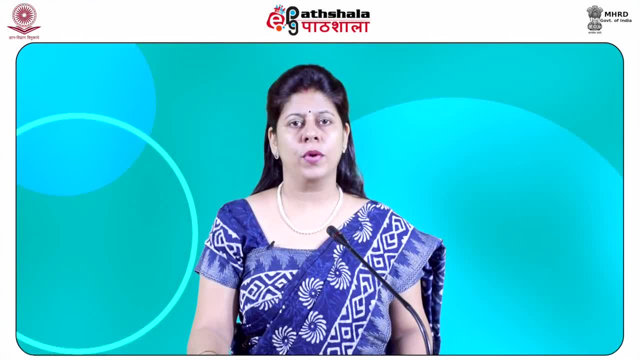 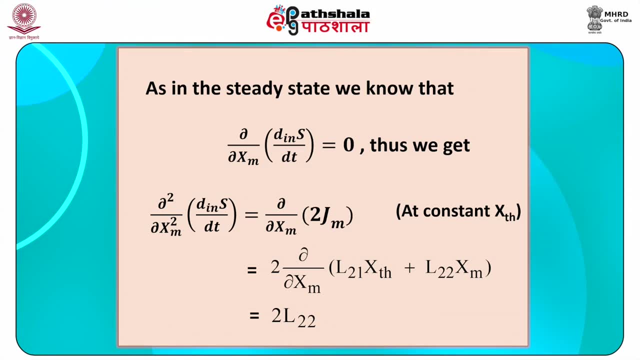 be shown by taking the second derivative of equation 19.. As in the steady state, we know that the differential of internal entropy with respect to Xm is equals to zero, we get finally twice of L22.. Since the sum is equal to two times the �m, we будет get its coefficient equals to 0.. 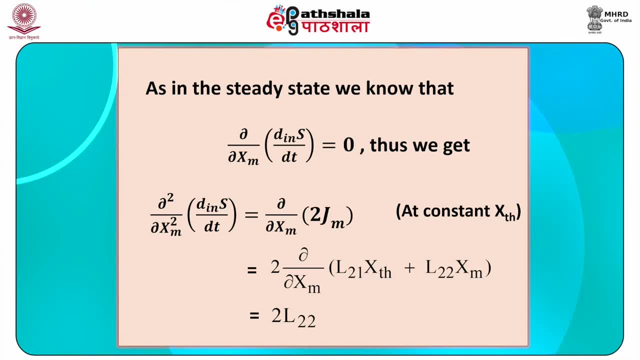 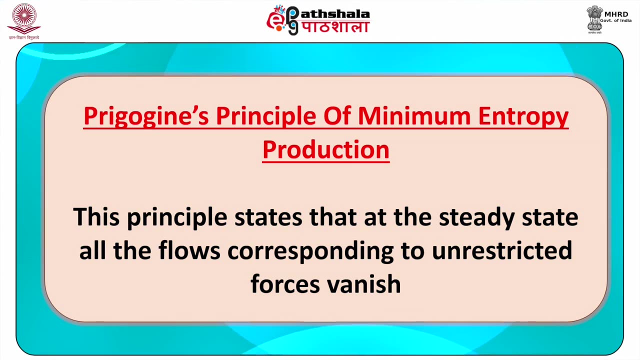 Since L22 has a positive value. thus the second derivative is also positive, so that the extremum is a minimum. This statement also furnishes the statement of Prigogine's principle of minimum entropy production. This principle states that at the steady state, all the flows corresponding to unrestricted 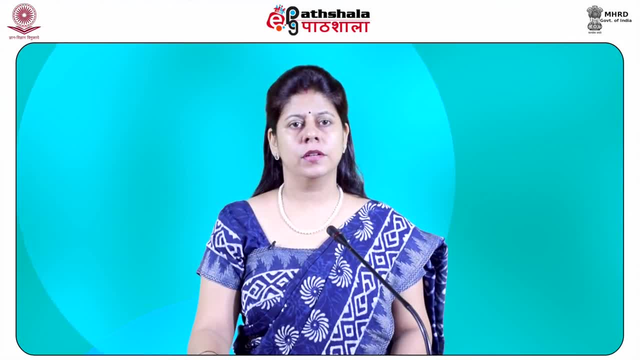 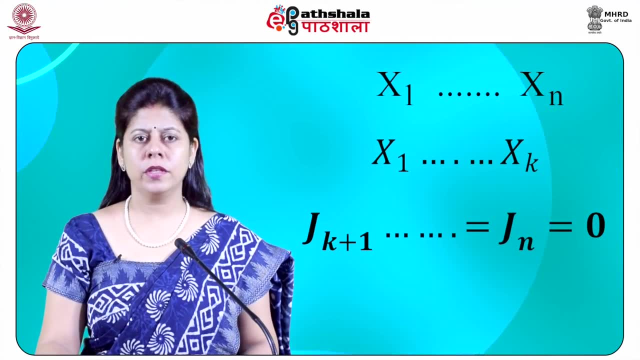 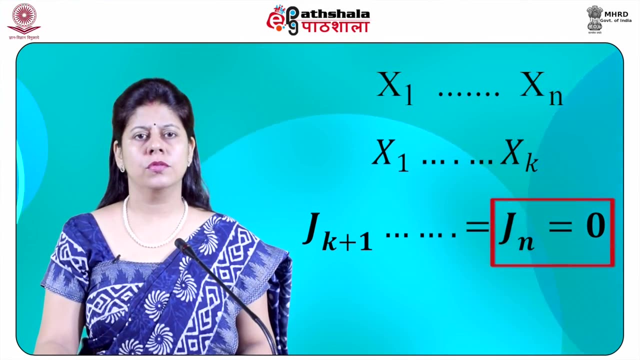 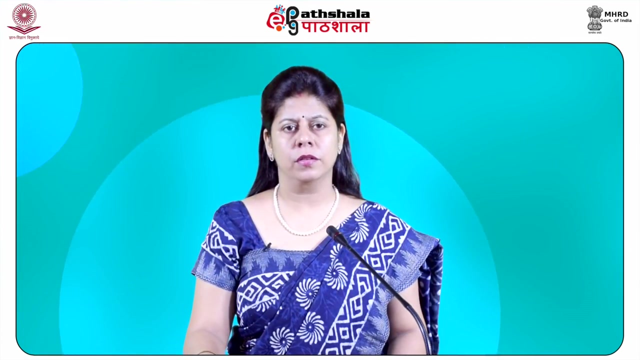 forces vanish. thus, in generalize, this can be generalized to the case of n independent affinities, out of which certain numbers are kept constant. For such stationary states, Jn is equals to 0. Such conditions are equivalent to minimum condition for entropy production, that is. 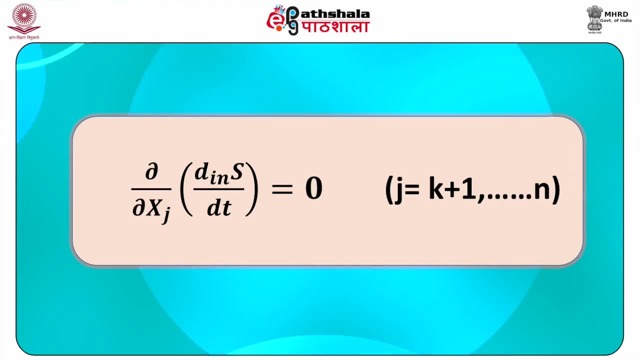 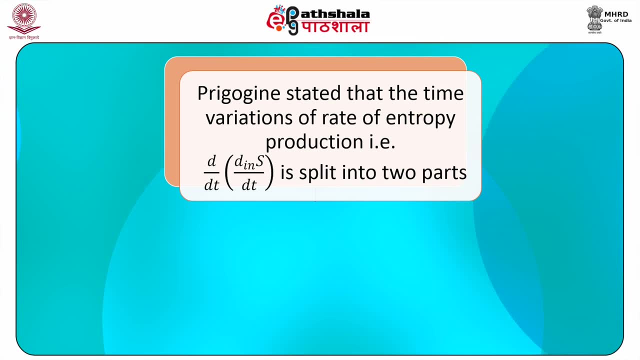 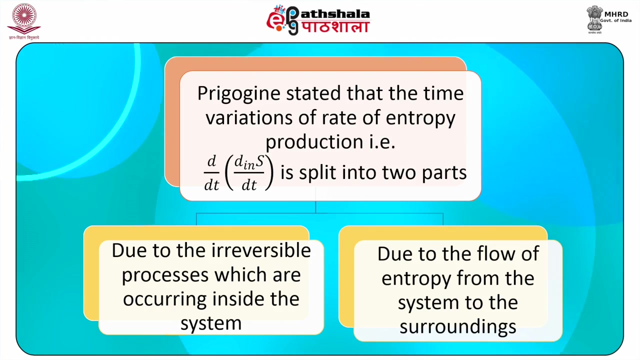 differential of internal entropy. with respect to xj. Prigogine stated that the time variation of rate of entropy production splits into two parts: first, due to the irreversible processes which are occurring inside the system and second, due to the flow of entropy from the system to the surroundings. Because of the irreversible processes occurring in the system. the rate of entropy production decreases Until the state is reached when it becomes minimum, when the system is in non-equilibrium steady state, then a system cannot come out of this state, despite being spontaneous, irreversible.